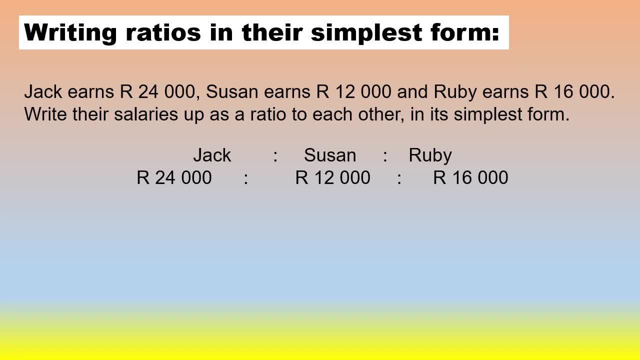 Jack to Susan to Ruby, 24,000 to 12,000 to 16,000.. So immediately can you see that you can eliminate three zeros from each number there to make it drastically smaller, without going to divide each one with a certain number and going again and dividing again. 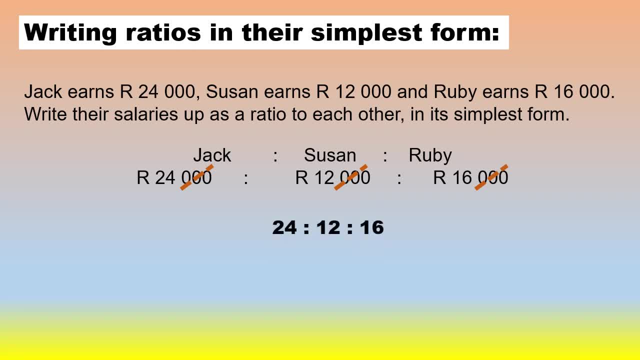 Okay, Then all right. so what is left? There's 24 to the ratio, 12 to the ratio 16.. Now, each of those numbers are even numbers, so I can easily divide them by two, which gives me 12 to the ratio, 6 to the ratio 8.. 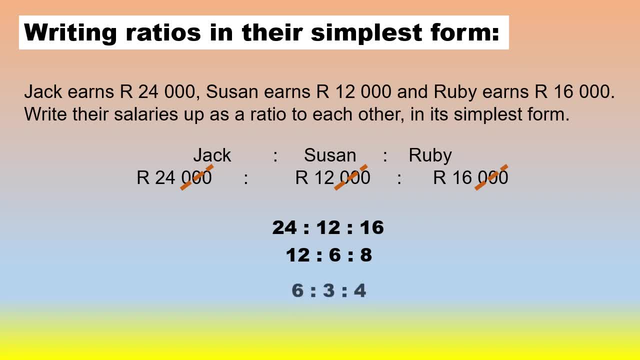 And again they're even numbers, so I can divide them again by two. and that leaves me with 6 to the ratio 3, to the ratio 4.. And that is its simplest form. All right, If you only have two ratios that you have to write in its simplest form, you're going to have to divide them by two. 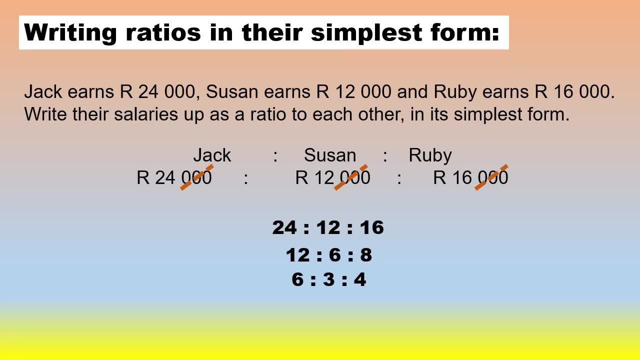 The easiest way to do that is you put it into your calculator. So if it is 12 to the ratio 16, you put it in as a fraction: 12 over 16, or 12 divided by 16.. Press your equal button and it will give you the simplest form on your calculator. 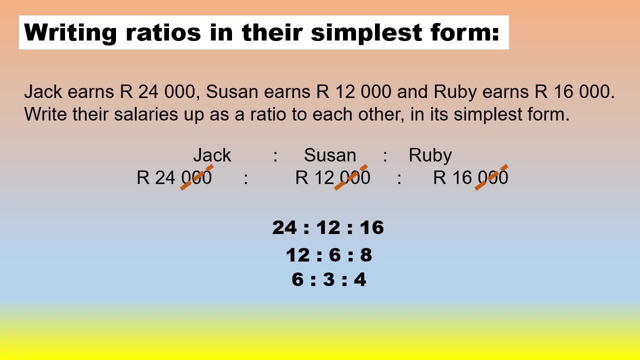 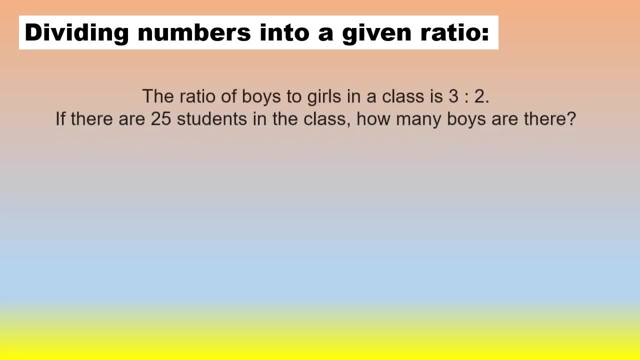 So you can also enter it as a fraction into your calculator. Okay, Let's have a look at another example, dividing numbers into a given ratio. The ratio of boys to girls in a class is 3 to 2.. If there's 25 students all together in the class, how many boys are there? 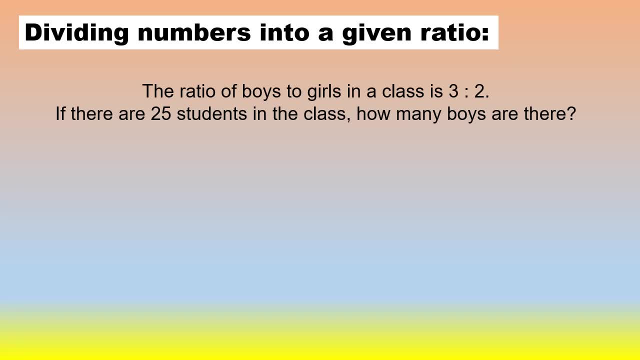 Now with this where they ask you, we'll do another one after this where you'll see if I say to you, if so many boys are there, how many girls are there. So with all of these type of questions, with a ratio, first things first is you want to write up your ratio: boys to girls, it's 3 to 2.. 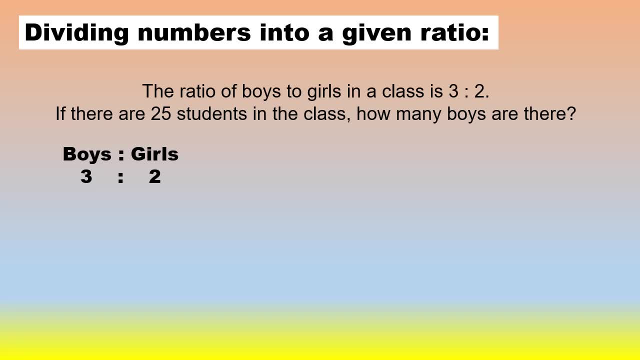 Then your next step is to calculate or to get the total number of parts that you are dealing with. So all you do is you say 3 parts boys and 2 parts girls. so 3 plus 2 is 5 parts all together. then. 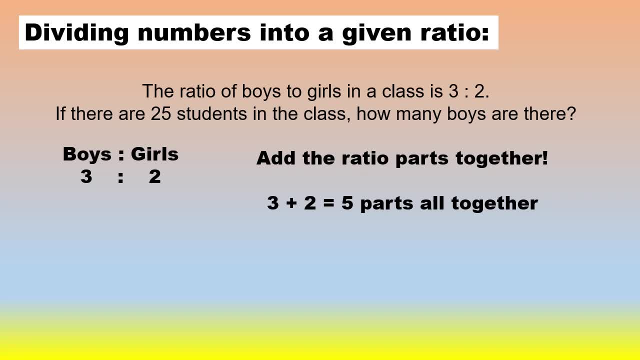 Okay. so you add the ratios together, 3 plus 2, and that would give you 5.. Now to work out the boys. you will say the boys are 3 out of the total parts, so 3 out of 5,. 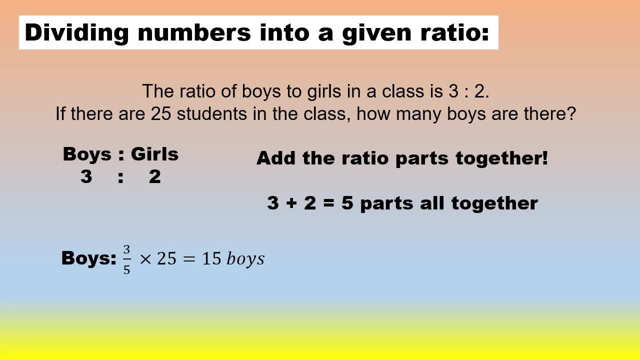 of the 25 are boys and of is a time sign. So 3 divided by 5 times 25 gives you 15 boys. Let's just pretend they also ask for the girls. Then you would say: for the girls it's 2 out of the 5 of the 25, and that gives you 10 girls. 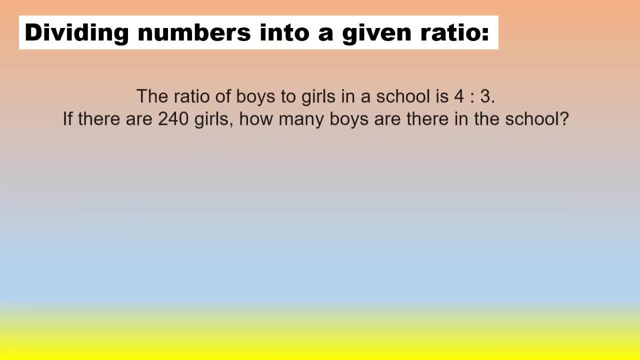 Right, let's have a look at another example. The ratio of boys to girls in a school is 4 to 3.. So if there are 240 girls, how many boys are there in the school? And with this one it's actually quite easy, because you don't have to add the parts together. 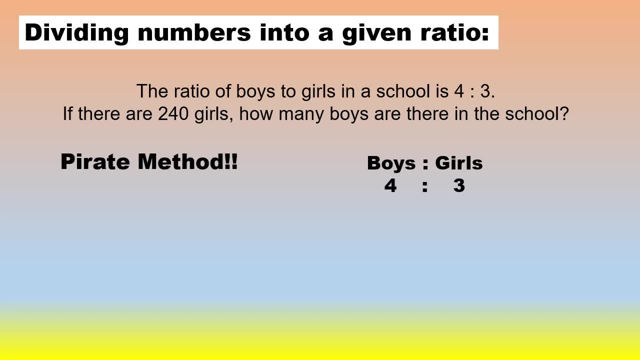 You're going to use the pirate method. Okay, so you write up: boys to girls is 4 to 3.. Underneath the girls you go and put 240. And then you know what to do. from there with the pirate method, You say 2 to 3.. 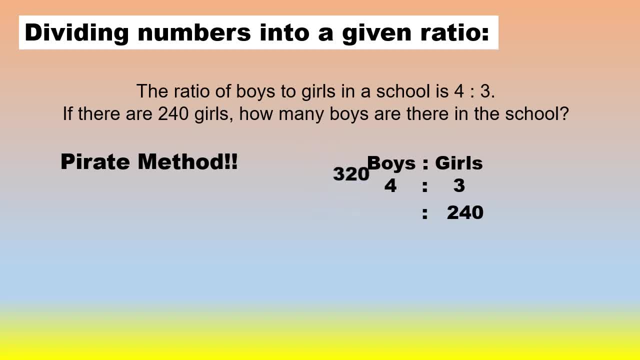 say, 240 divided by three times by four, and that gives you 320 boys. Another question they could have asked is how many students are there then in the school? And then you would have just said 320 plus the 240, and that's the total number of students. Okay, another example: Inheritance of 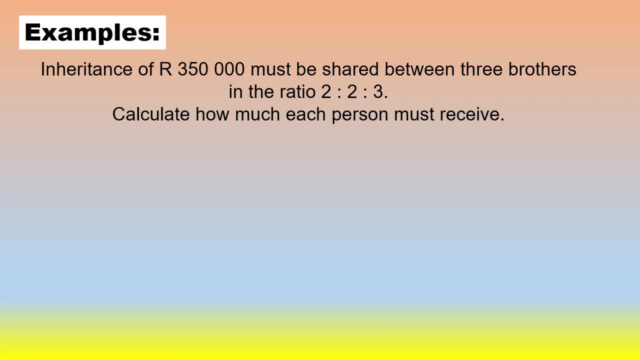 350,000 must be shared between three brothers in the ratio two to two to three. Calculate how much or how much each person must receive. Okay, so now, they didn't tell you the one person got this much. They say to you: basically divide 350,000 into the ratio two to two to three. The first: 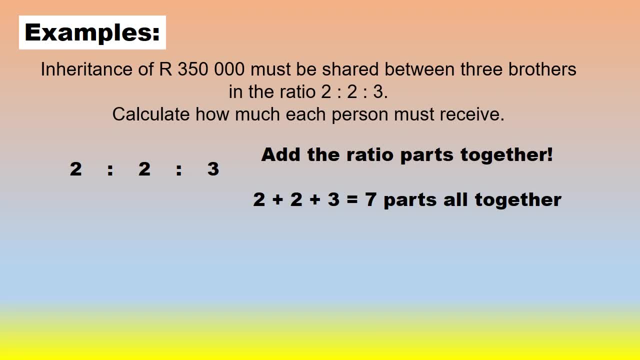 thing that we have to do is we have to add up all the ratio parts together. So two plus two is four plus another three gives you seven parts all together. So person number one, he got two parts, Two out of the seven parts of the 350,000.. Okay, so two divided by seven times 350,000 gives you. 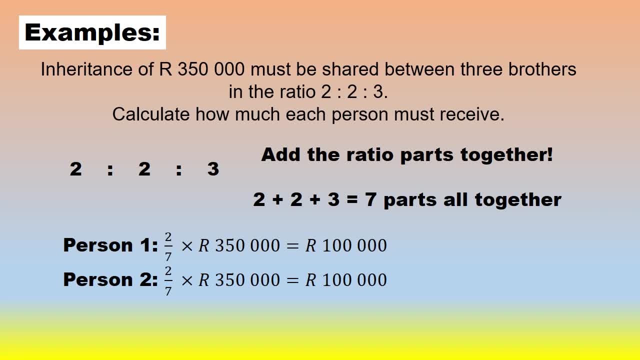 100,000.. Same with person two. He also got two parts. Two parts out of the total seven parts also gave you 100,000.. And person three- maybe he was the favorite, So he got three parts. Three out of the seven times the 350,000 gives you 150,000. 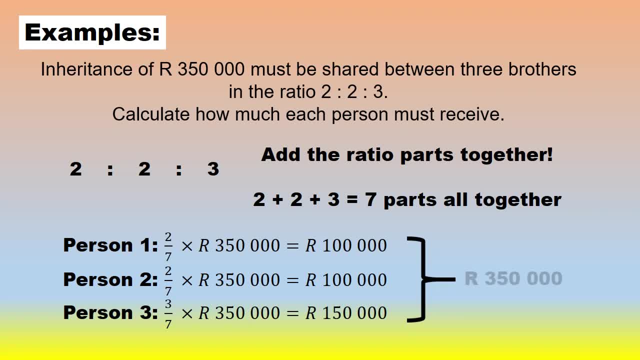 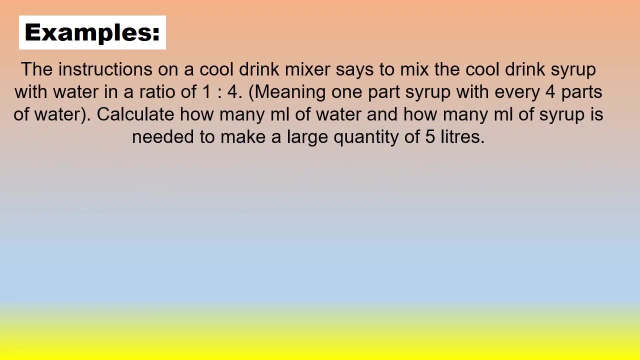 At the end. what you can do to just make sure is add all your answers together and it should give you the total part of inheritance again of 350,000.. Okay, let's have a look at another example. Maybe this illustrates it a little bit better for you- all the different parts, why we have to add them. 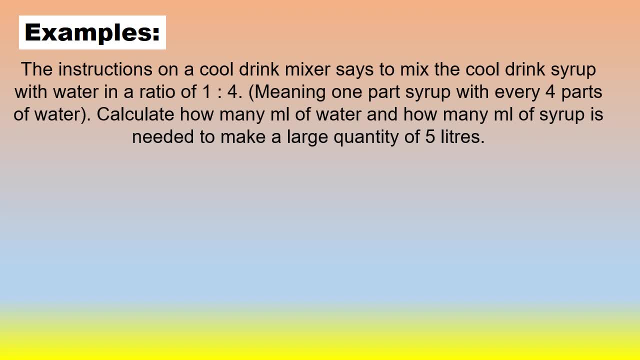 together. The instructions on a cool drink mixer says that to mix the cool drink syrup with water in a ratio one to four, Meaning one part syrup or cool drink- Either. you want to say it- with every four parts of water. So calculate how many milliliters of water and how many milliliters of syrup is needed to make a large. 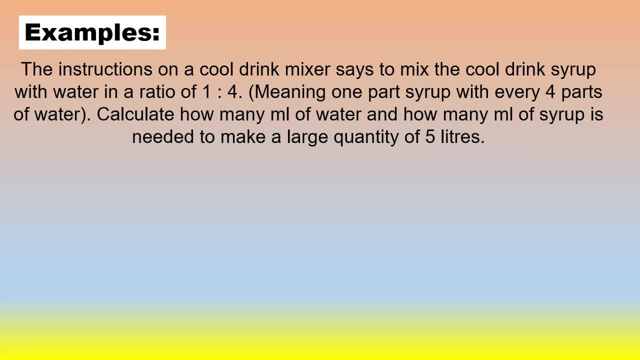 quantity of five liters. Okay, so you want to make five liters of cool drink. but they ask you very carefully, have a look. They say how many milliliters of each do you need? So if you think of five liters, how many milliliters in a liter? A thousand? 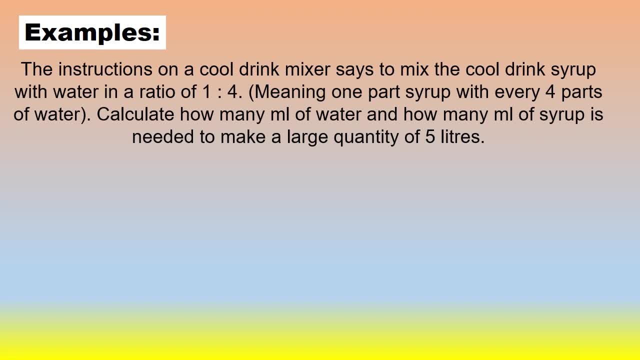 Five thousand milliliters. That is what you want to make, All right, so let's have a look, Let's represent that as our glass. And then we've got one part syrup with one, two, three, four parts water. Okay, so sorry, let's think of that as a huge container, because we want to make five liters. 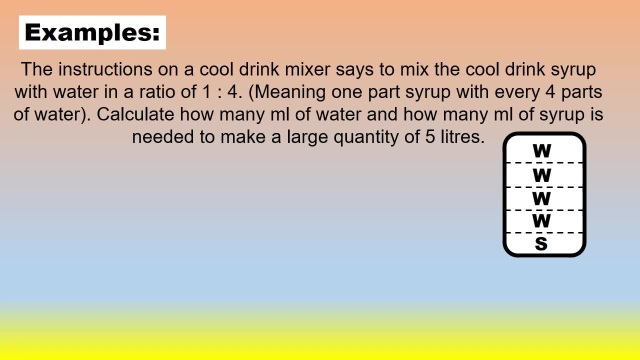 of it. So one part syrup with every four parts of water. So if you add it all together to make a full can, full of juice or cool drink that you are making, can you see that it's one, two, three, four, five parts all together And that is why it's very important to add your ratio parts together.